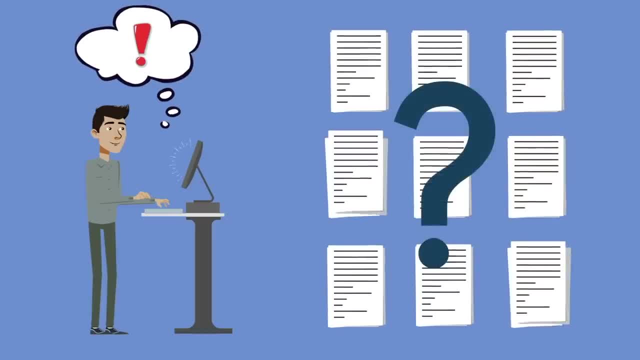 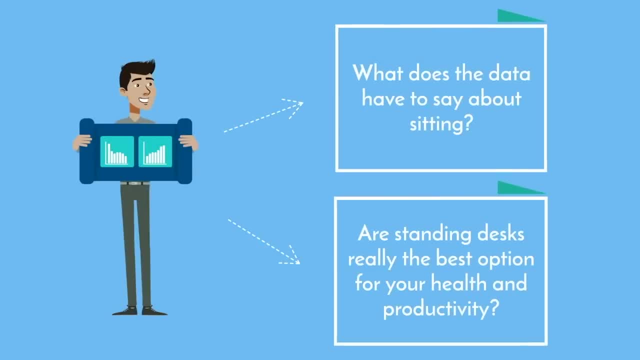 I found myself surprised, as the data isn't as clear-cut as some would have you believe. So what does the data have to say about sitting, and are standing desks really the best option for your health and productivity? First, it's important to understand the arguments against sitting and traditional. 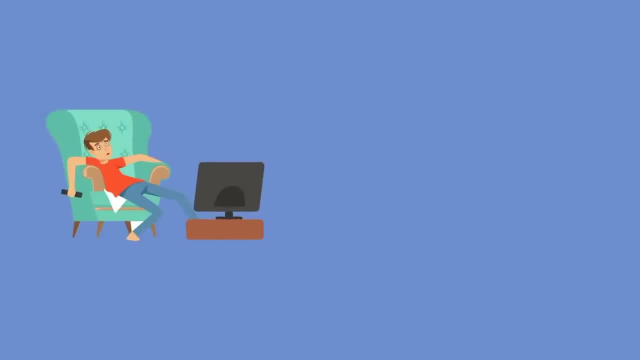 desks. So what's so bad about sitting? Well, the fundamental principle is that a sedentary lifestyle and the physiologic changes that ensue are the same. So what's so bad about sitting? Well, the fundamental principle is that a sedentary lifestyle and the physiologic changes that ensue are the same. 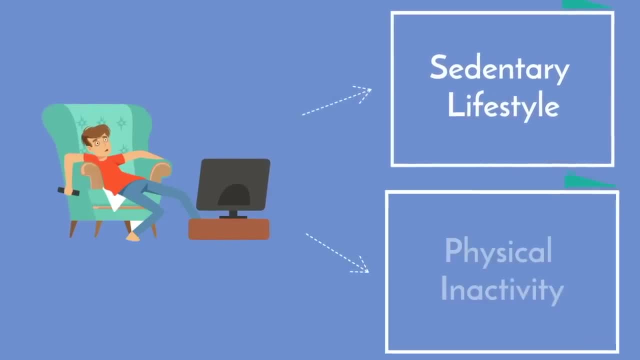 So what's so bad about sitting? Well, the fundamental principle is that a sedentary lifestyle and the physiologic changes that ensue are the same, And there's a lot of evidence that physical inactivity is linked to higher morbidity and mortality. but the question is how this relates to sitting. 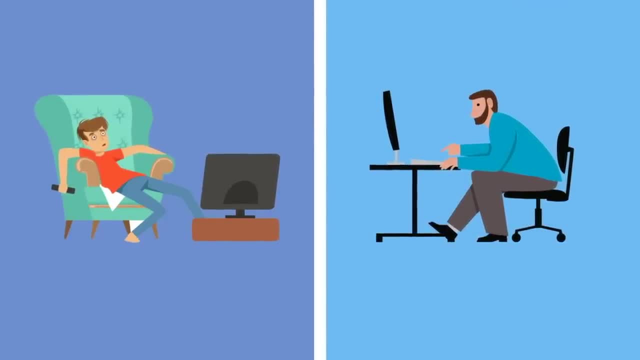 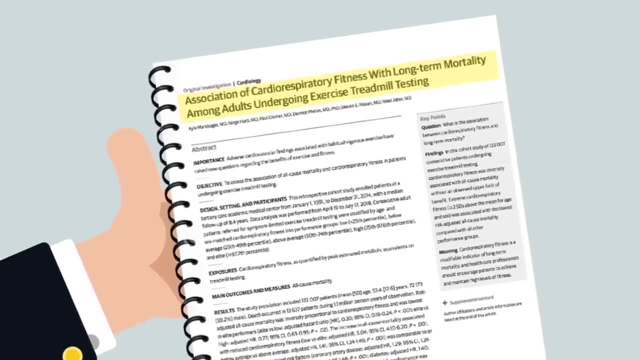 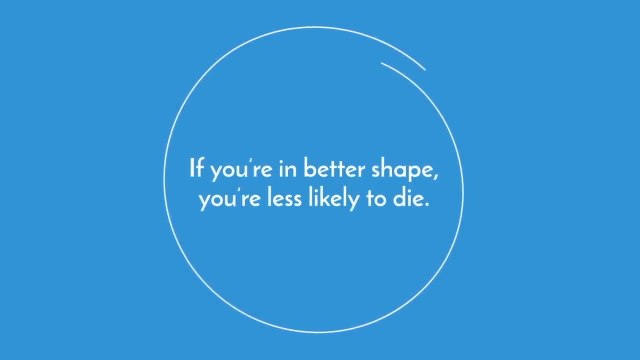 at our desks And whether standing desks are a viable alternative. Mandsager and colleagues demonstrated in 2018 that poor cardiorespiratory fitness, as assessed on an exercise treadmill test, was strongly correlated with mortality. In short, if you're in better shape, you're less likely to die. It's important to note, however, there's 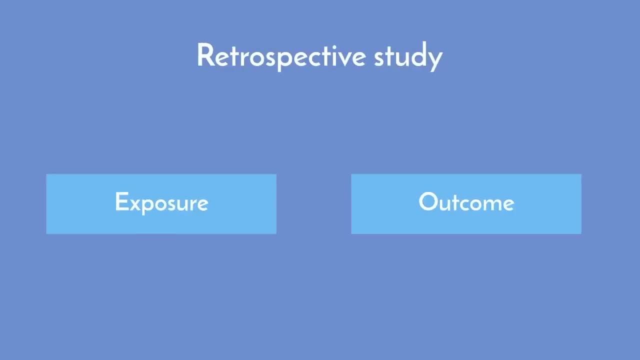 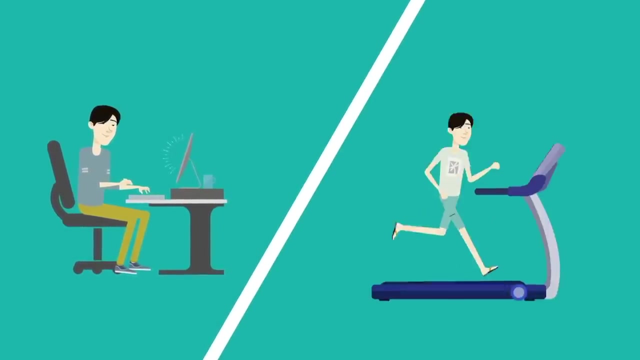 that this study and many others are retrospective studies and therefore, by definition, they demonstrate correlation not causation. Additionally, it's been noted that the negative effects of sitting aren't reversed by exercise, Reason being the metabolic changes and subsequent deleterious effects induced by sitting aren't. 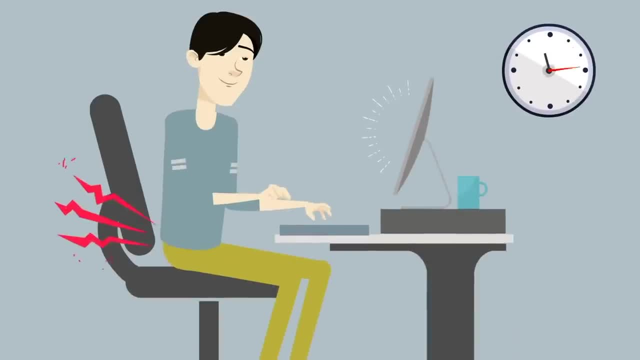 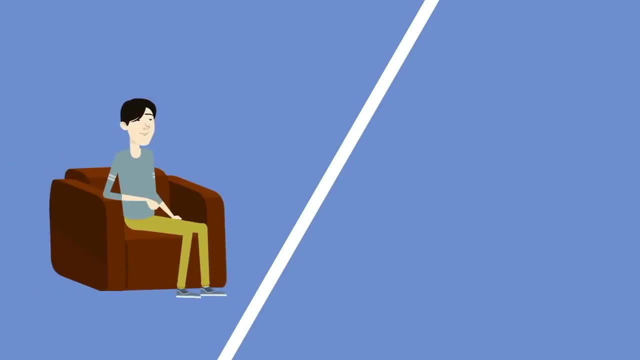 simply reversed by being active. Sitting also increases the pressure to your lower back in comparison to standing. Ever notice that your back hurts more when you sit for prolonged periods of time. So let's talk about the evidence for standing desks Now. if sitting for prolonged periods is bad for us, it's easy to see how standing desks 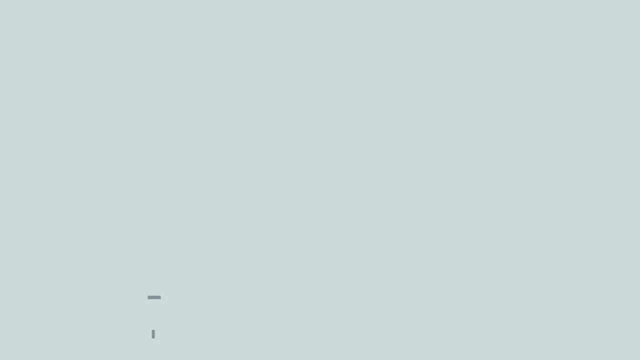 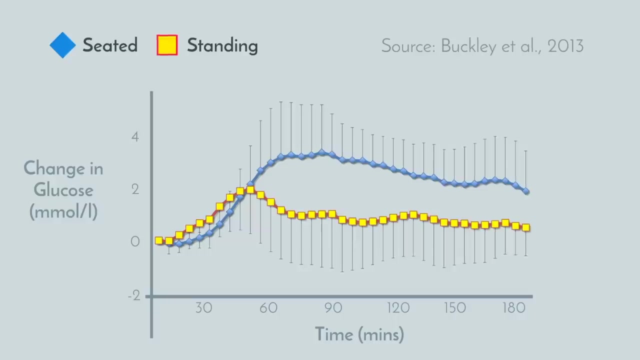 would seem like a logical solution. In 2013,, Buckley and colleagues demonstrated that standing reduces postprandial glycemic variability, meaning your blood sugar varies less after eating a meal if you're standing. This is good as greater amplitudes of glycemic variability. 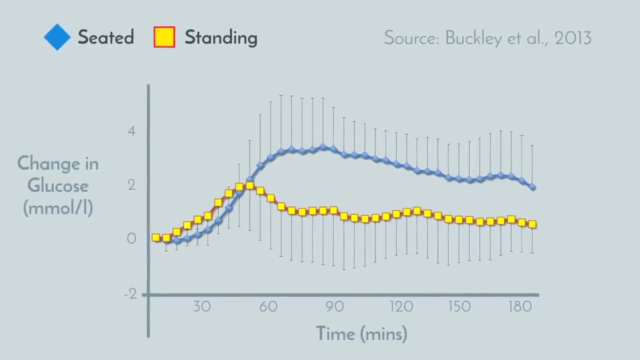 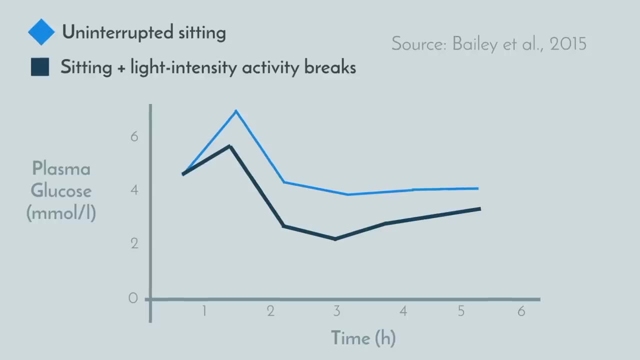 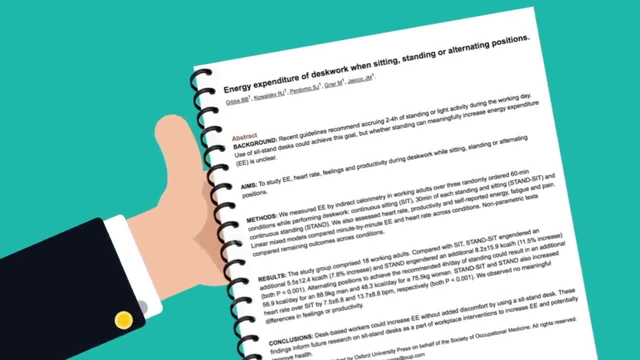 have been linked to circulatory oxidative stress. However, Bailey et al in 2015 had conflicting data suggesting that standing did not alter postprandial glycemic variation, but short bouts of light intensity activity did. In 2017, Gibbs and colleagues postulated that decreased caloric expenditure could be a specific 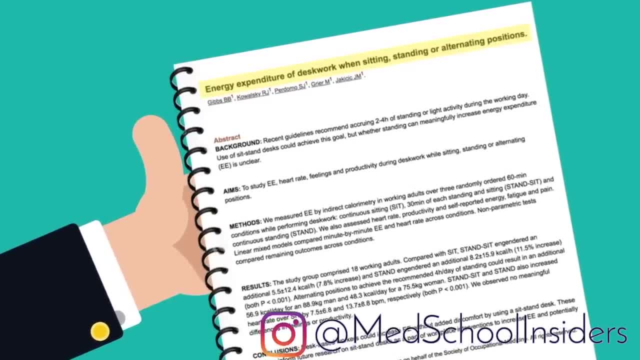 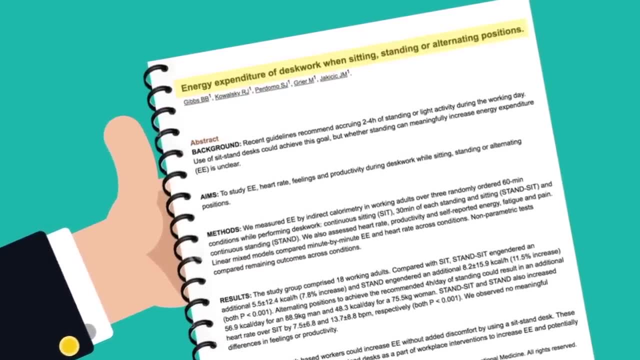 mechanism through which sedentary behavior increases health risks, such as by contributing to an energy imbalance leading to obesity. They also demonstrated that sitting for prolonged periods of time increases the risk of obesity. They also demonstrated that standing expends more energy than sitting. 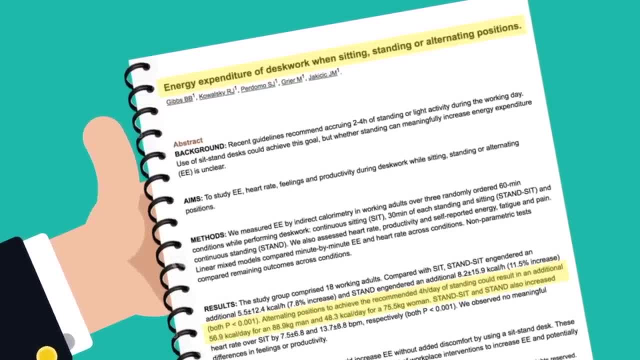 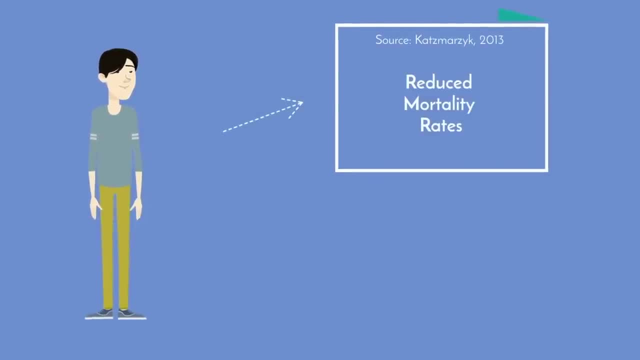 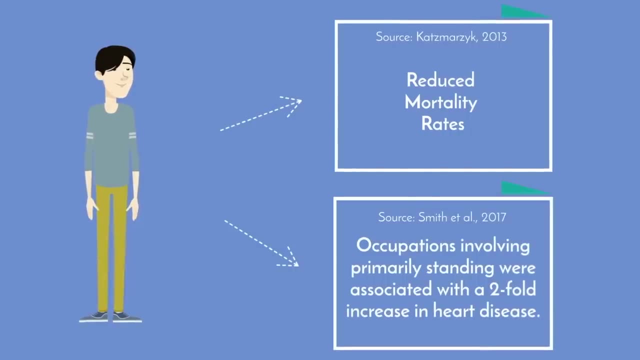 No surprises there. As a whole, however, the literature regarding the benefits of standing desks is not clear-cut. Katzerczyk in 2013 suggested that increased standing time was correlated to reduced mortality rates, but Smith and colleagues in 2017 suggested the exact opposite, that occupations involving 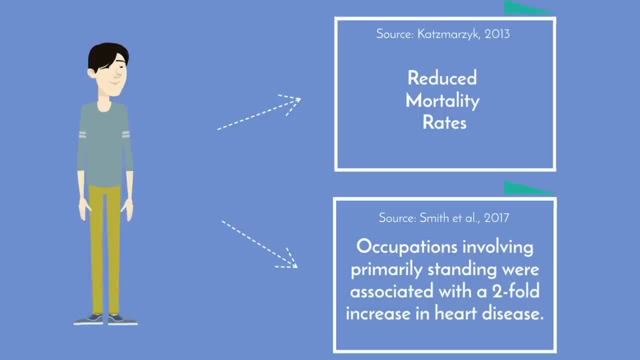 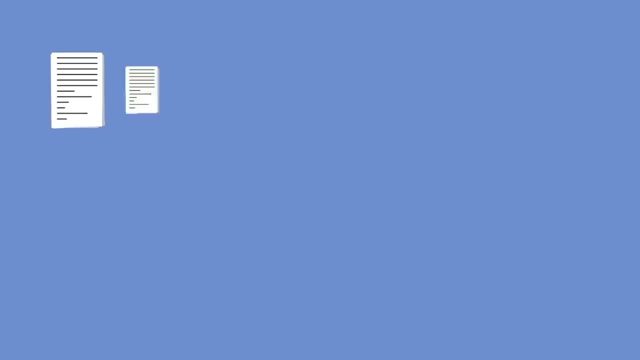 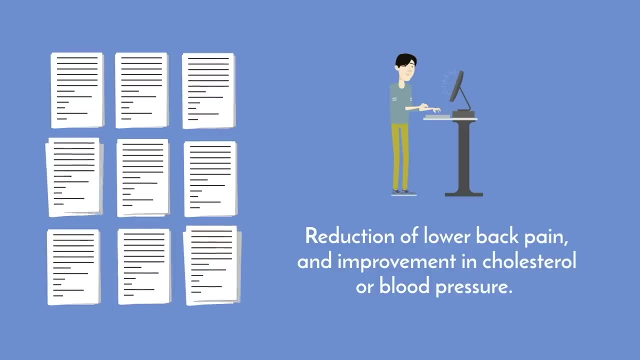 primarily standing were associated with a two-fold increase in heart disease compared to occupations involving predominantly sitting. Several other studies I came across in my research emphasized the increases in physical activity associated with standing desks: reduction of lower back pain and improvement in cholesterol or blood pressure. 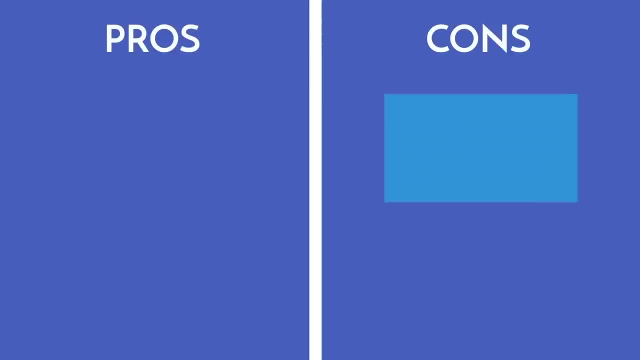 However, others suggested that increased physical activity at a standing desk was offset by a decrease in physical activity away from the desk, And while some studies pointed to improvements in psychological well-being, creativity and no detrimental effects to focus or productivity, others concluded that standing desks were 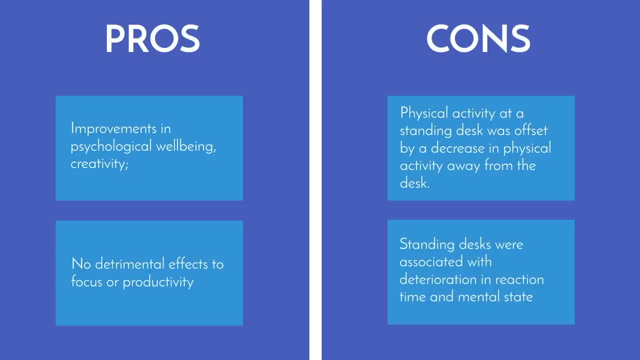 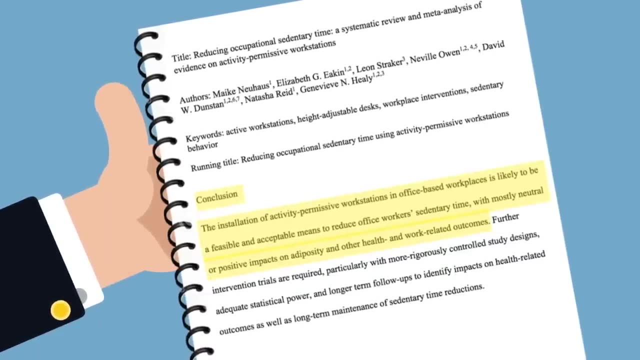 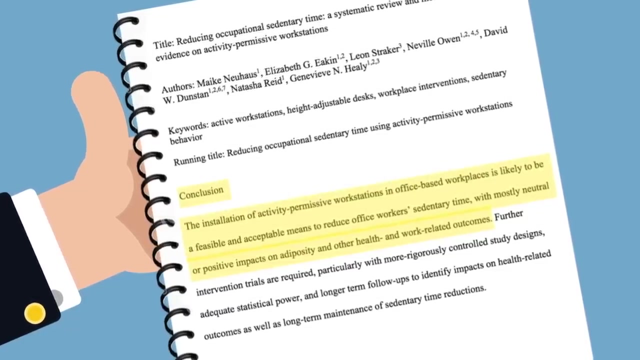 associated with a deterioration in reaction time and mental state. The data is best summarized by two systematic reviews In 2014,, Newhouse and colleagues concluded that the installation of activity-permissive workstations in office-based workplaces is likely to be a feasible and acceptable means. 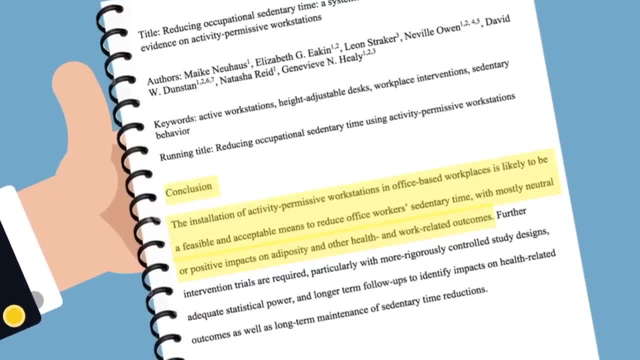 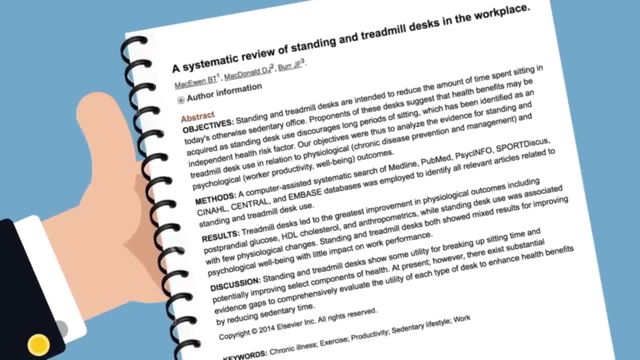 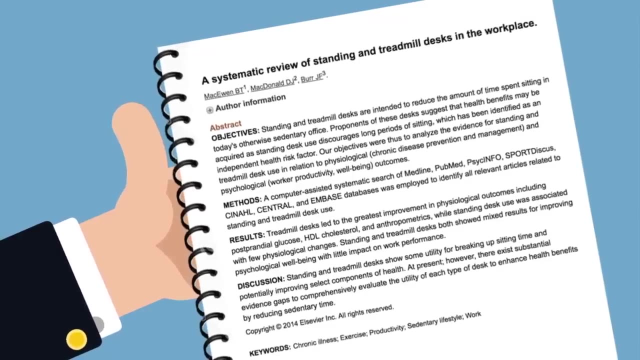 to reduce sedentary time, with mostly neutral or positive impacts on adiposity and other health and work-related outcomes. The systematic review by McEwen and colleagues in 2015 concluded that there wasn't enough evidence to evaluate the utility of each type of desk. however, treadmill desks demonstrated. 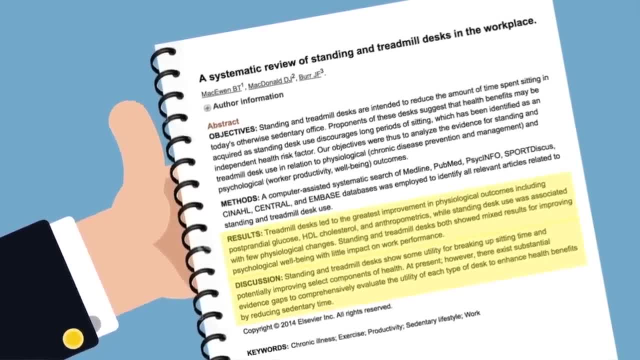 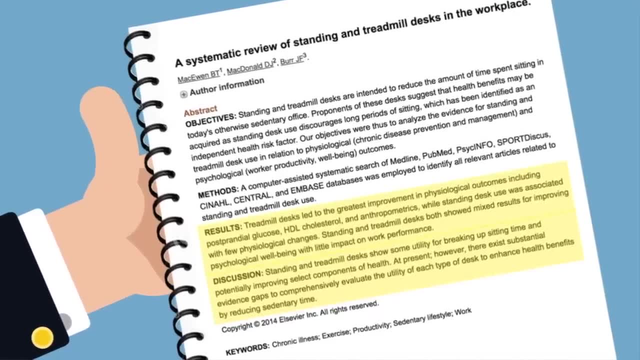 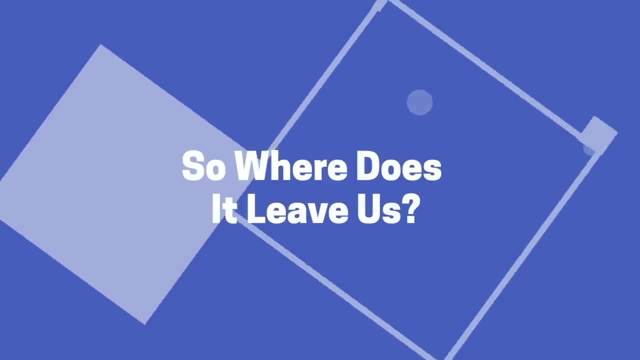 the most significant improvements in glucose, cholesterol and fat loss. Standing desks had few physiologic changes, but improved psychological well-being And ultimately, too much standing or sitting would result in discomfort. So where does it leave us? The key takeaway from my deep dive in the literature is that the literature on standing 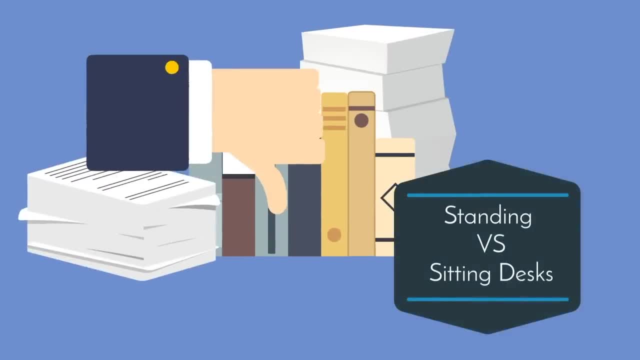 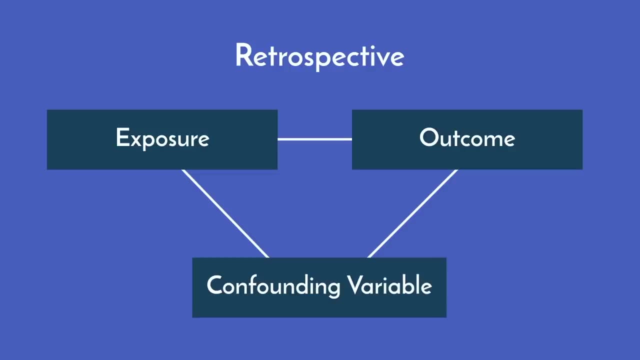 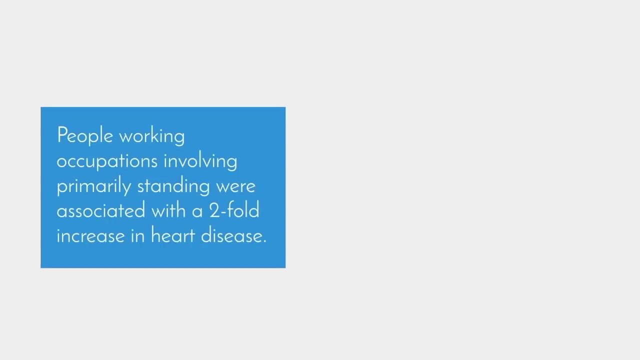 versus sitting desks kind of sucks. The overwhelming majority of studies were retrospective and did not adequately control for possible confounding variables. For example, Smith and colleagues demonstrated that people working occupations involving primarily standing were associated with a two-fold increase in heart disease, But without controlling for the type of occupations, socioeconomic variables and other demographic 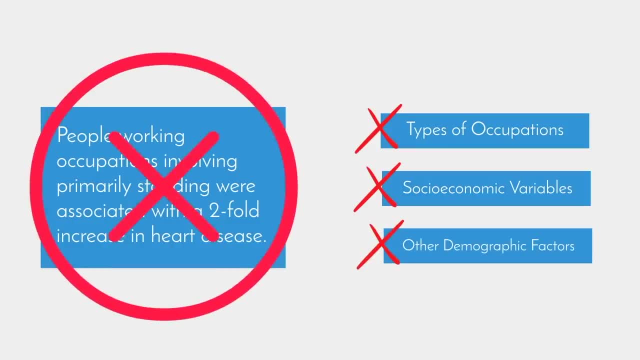 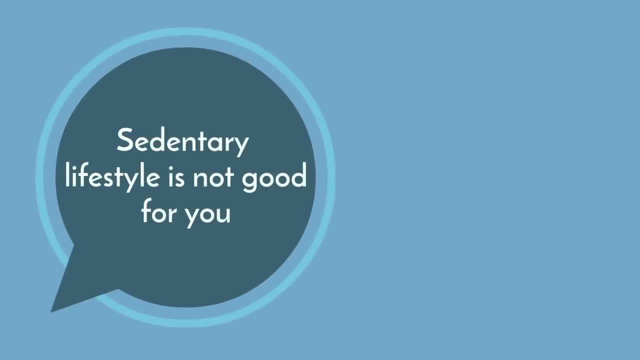 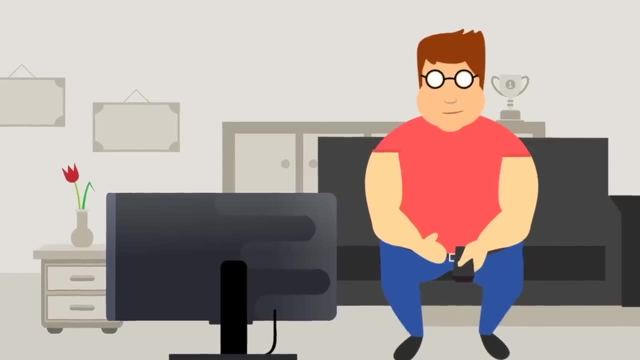 factors, All of that information is close to meaningless. The data is quite strong, though, that a sedentary lifestyle is not good for you, But I'm not convinced that a standing desk is necessarily the solution. This is a complex problem. people are no longer getting much exercise in their lives and 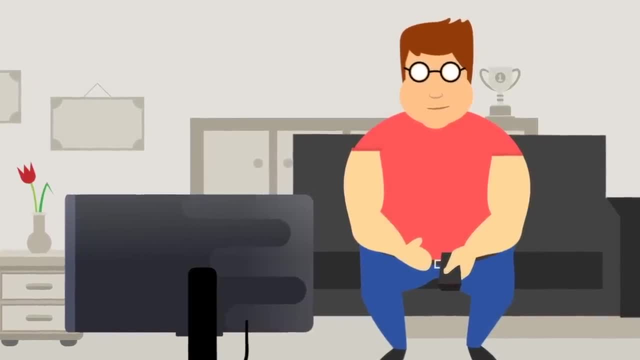 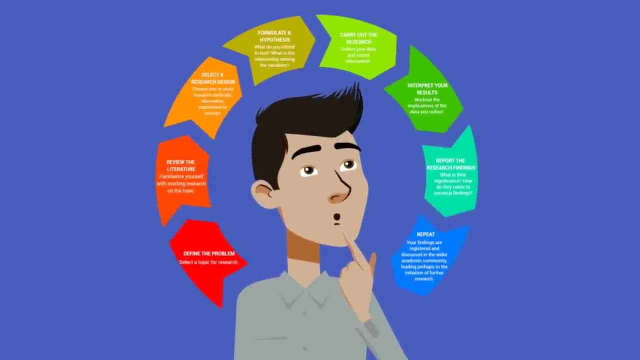 we are proposing an incredibly simple solution, hoping it's an easy fix. Unfortunately, even with the scientific method, we don't get clear-cut answers And we must make decisions with imperfect information. So should you sit or should you stand at your desk? 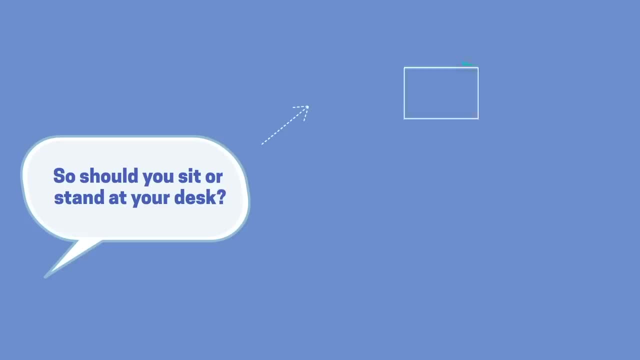 I would argue that isn't the right question to ask. In 2018, Caldwell and colleagues even demonstrated that prolonged standing resulted in measurable increases in arterial stiffness. That's not good. It means, then, that any form of inactivity, whether while standing or seated, results. 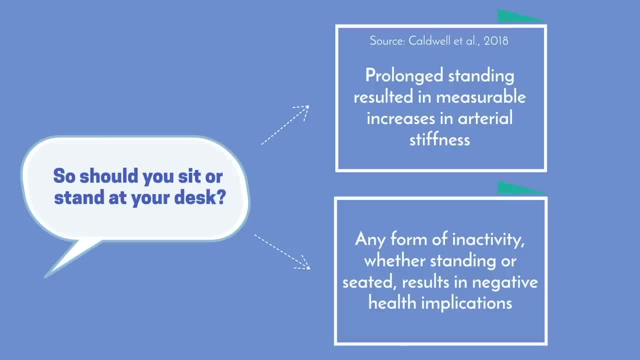 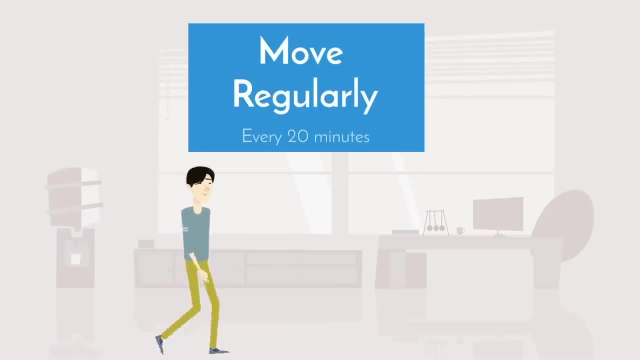 in negative health implications. Instead of focusing on standing versus sitting at our desks, it appears that the most important principle is to move. Move regularly. Some have suggested every 20 minutes as a good rule of thumb. Our bodies are designed to move. 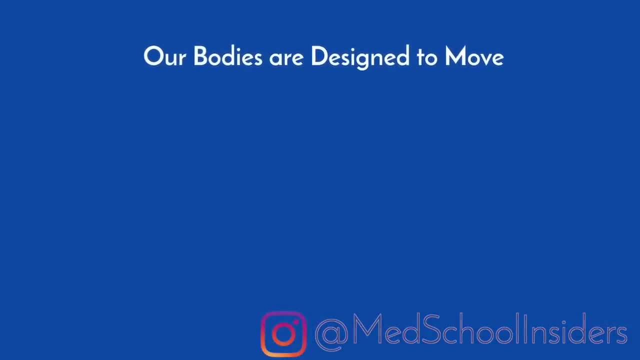 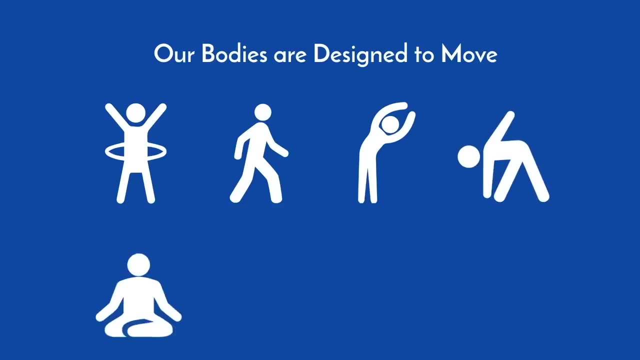 We aren't designed to sit still, So even if you're using a standing desk, you don't want to stand immobile all day. You should be shifting, walking, moving, stretching, doing yoga poses and switching between sitting and standing throughout the day. 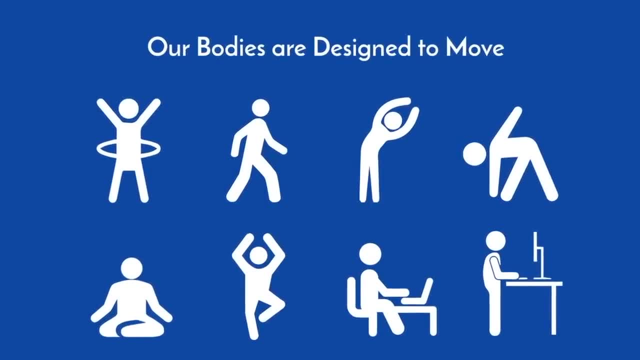 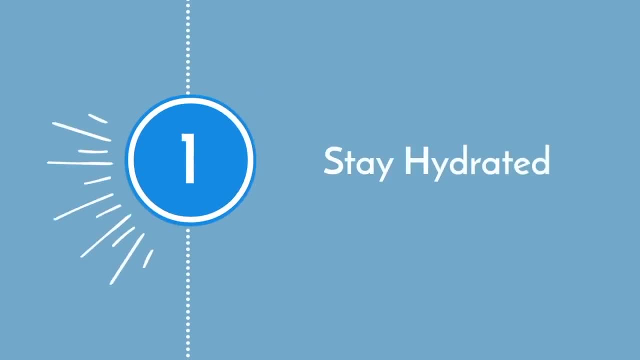 But because this is Med School Insiders, I don't want to leave you hanging. I want to give you some actionable advice. Here are three points to act on. First, stay hydrated. One of my favorite methods to induce movement is to stay well hydrated. 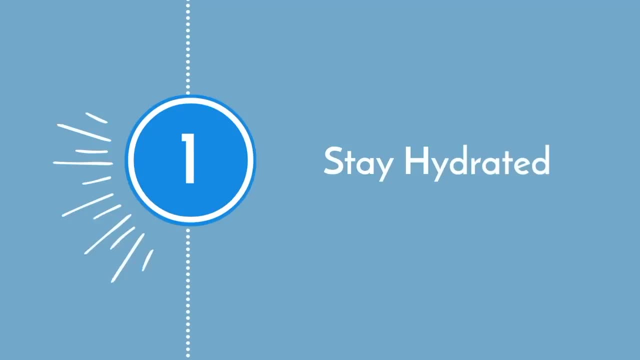 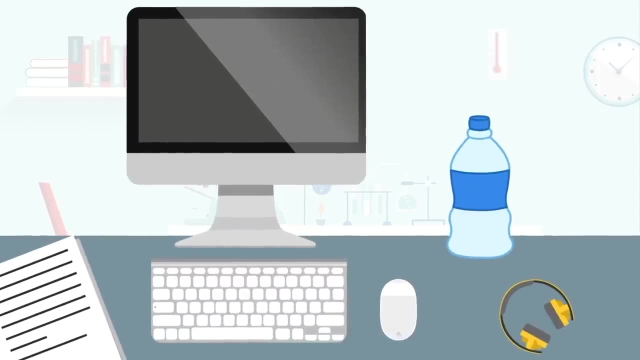 It has the benefit of well keeping me hydrated, but also the side benefit of prompting me to move regularly, as I need to use the restroom frequently. If you need a friendly reminder to drink more water, the easiest thing you can do is to: buy a water bottle and keep it nearby. I personally opt for the BPA-free Nalgene 1.5L. I bought it for $10.00.. It was $10.00 over five years ago and it's still serving me well. 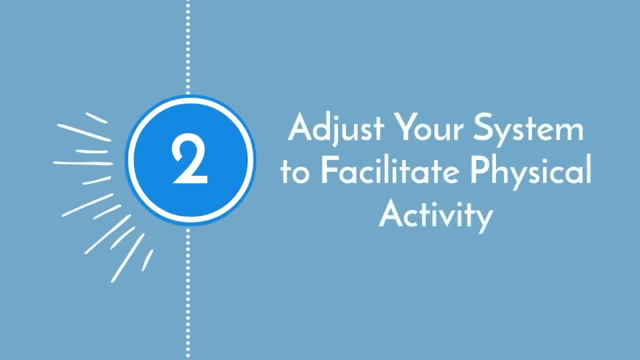 Link in the description below. Number two: adjust your system to facilitate physical activity. Remember that your systems produce results. After watching this video, if you feel motivated to move and exercise more, I guarantee it won't last. If, instead, you take that motivation and use it to change your systems, you'll be much.